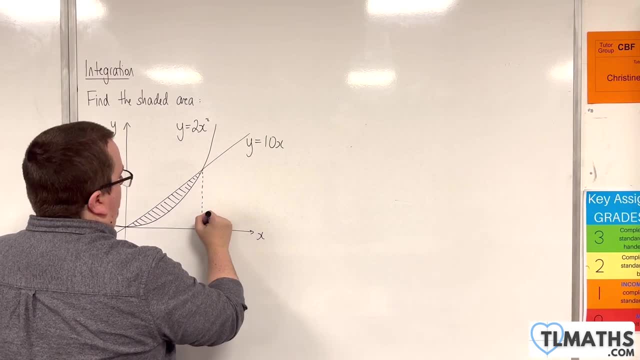 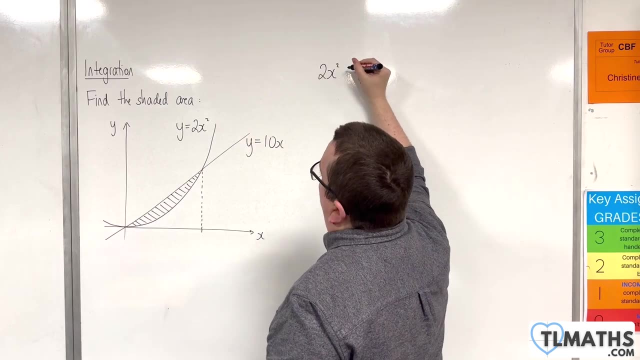 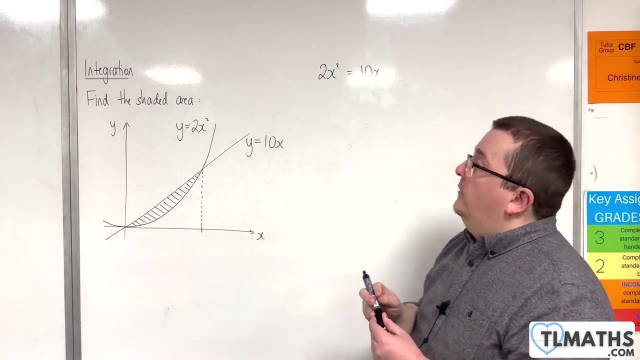 So we need to work out this point here, okay, before we continue. So to do that, I'm going to put the curve: y equals 2x squared equal to the line. y equals 10x. So 2x squared is equal to 10x. Now I'm going to divide through by 2 and move everything onto the left hand side. 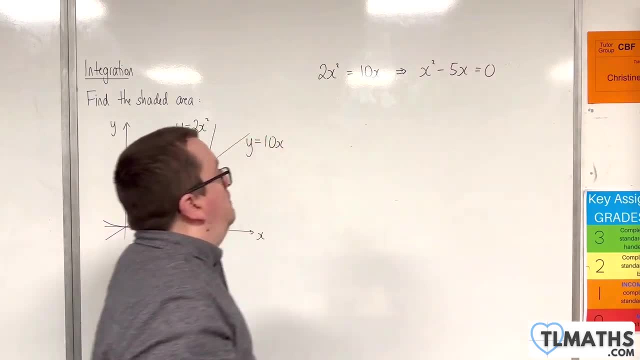 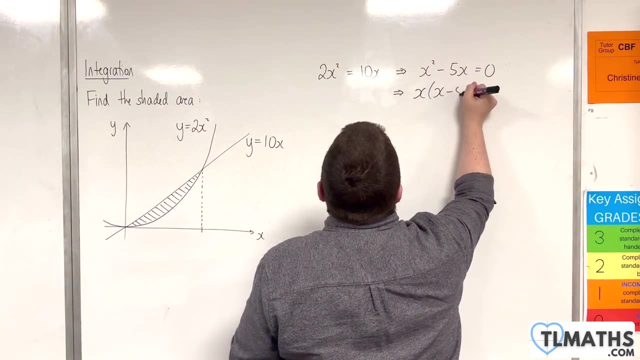 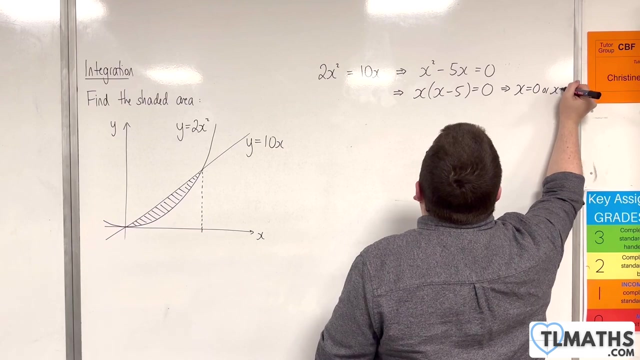 So I'm going to get x squared. take away 5x is equal to 0.. Now that quadratic can be factorised. So x, x, take away 5 is equal to 0. So that's telling me that x is 0 or x is 5.. 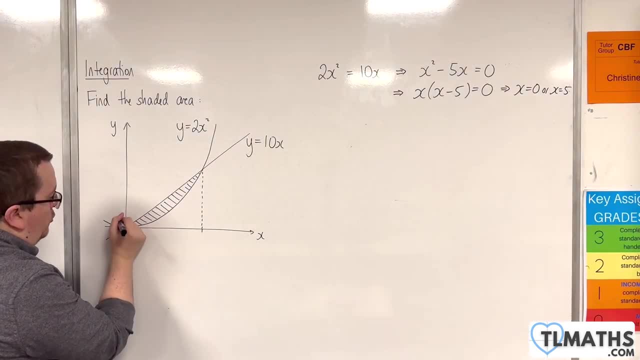 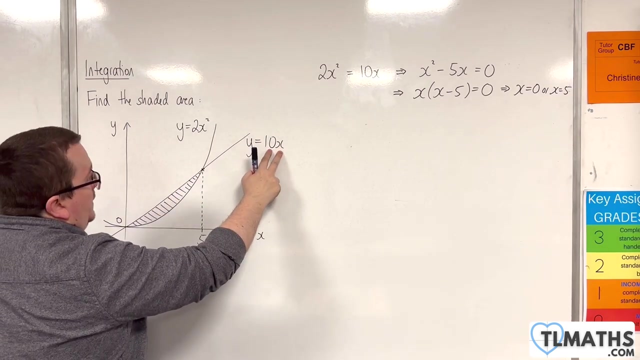 So the two points of intersection are at 0, so at the origin and here at 5.. Okay now, because that x value is 5, this point here must have coordinates of 5 and then 50.. So 5, going into that 10, lots of 5, is 50.. 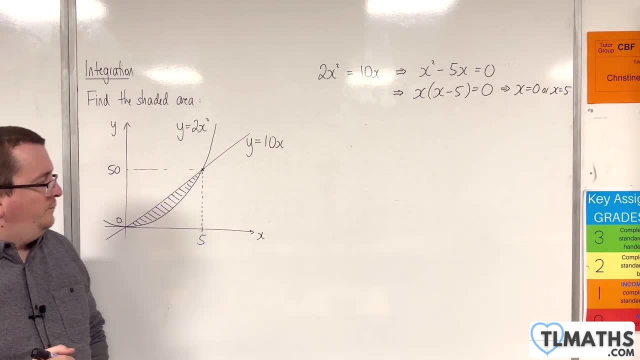 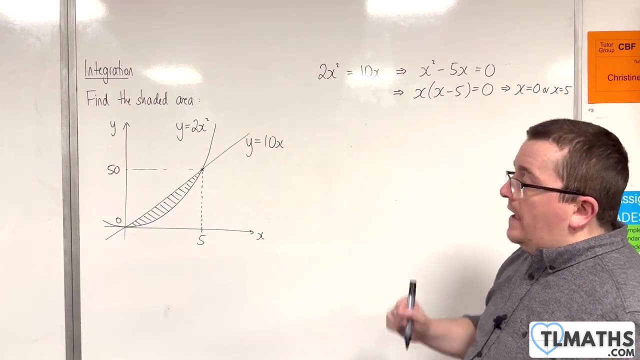 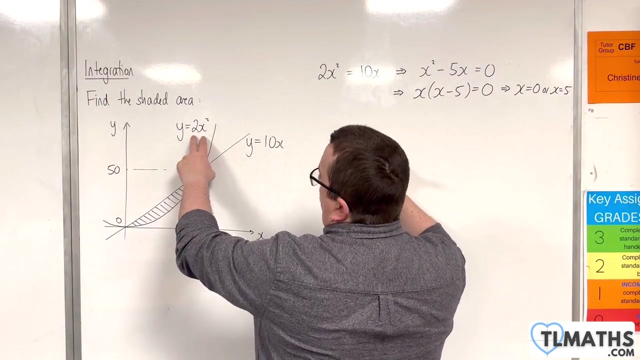 That's 50 there, okay. So we know that integration allows me to find the area between the curve and the x-axis. So if I was to find the integral of 2x squared between 0 and 5, what that would do is it would give me all of this section. 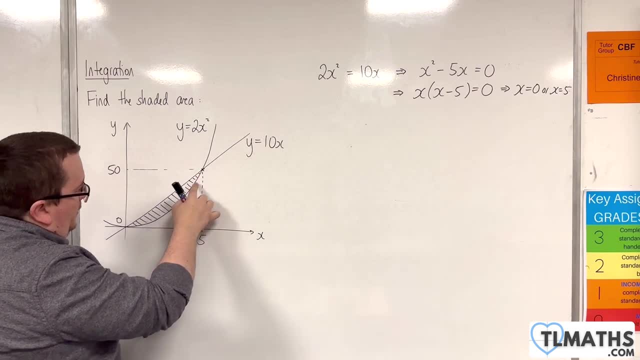 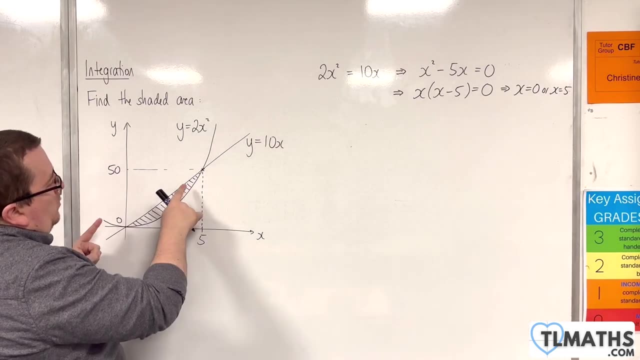 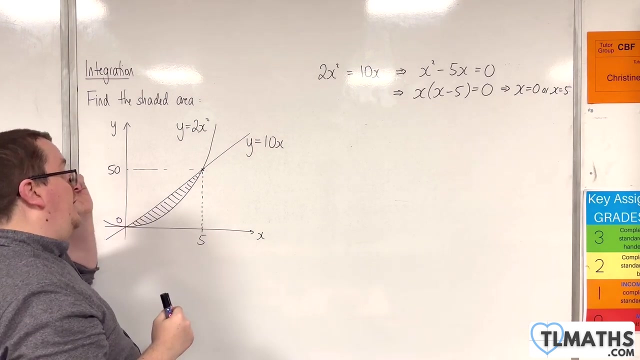 Okay, so this section here underneath the graph, but between the x-axis, Between the curve and the x-axis. Now what we need to do to work out the shaded area is: subtract that away from the area of the triangle. Now you can work out the area of the triangle in two ways. 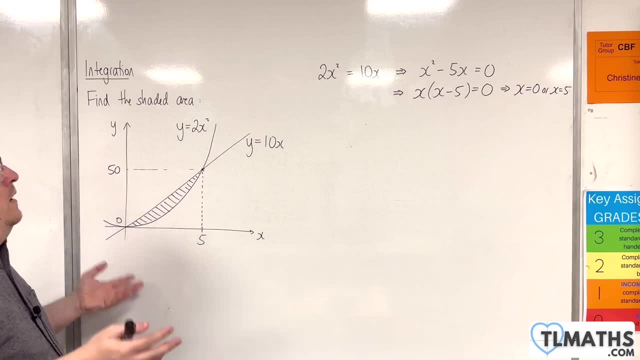 Either you do half base times height, which is going to be the easier way, Or you can integrate the line between 0 and 5. That will give you precisely the same result, But for these types of problems you should be looking, Looking out for triangles, rectangles, and then utilising that. 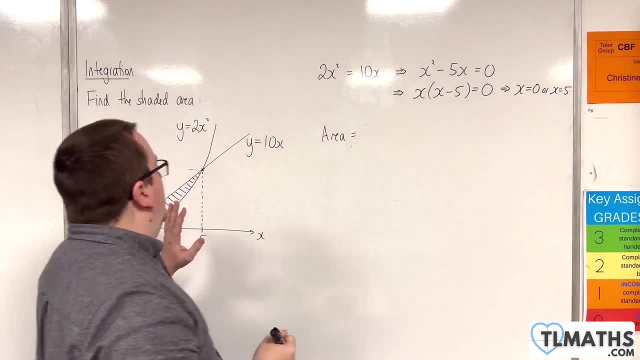 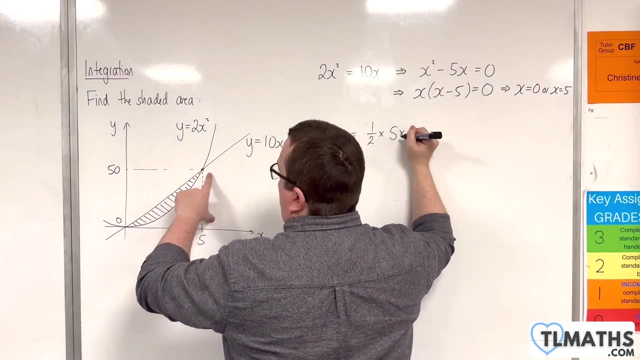 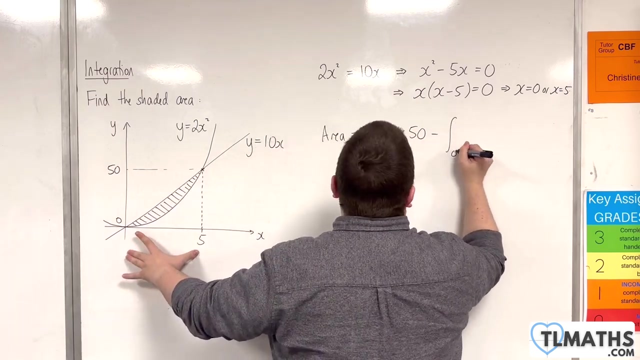 It's a lot quicker. So I'm going to work out the area of the triangle Which is going to be one half times the base, which is 5 times by the height, which is 50.. And then I'm going to take away the integral between 0 and 5 of the curve: 2x squared dx. 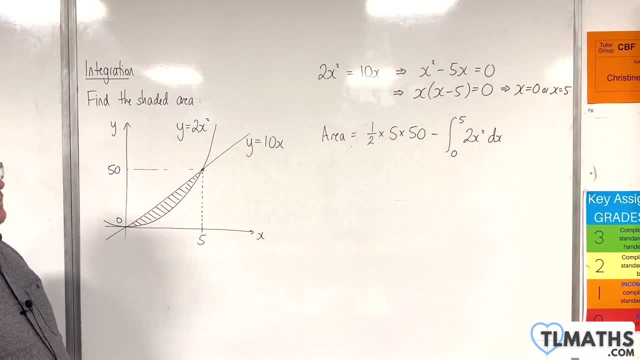 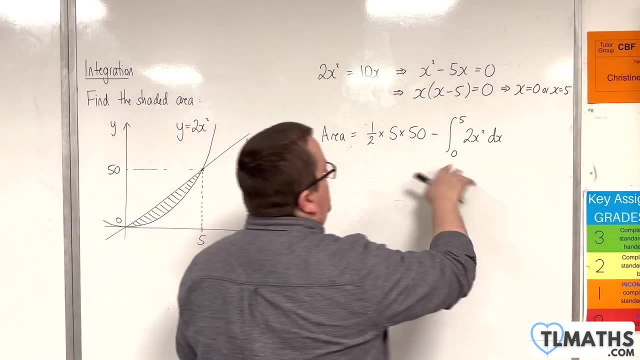 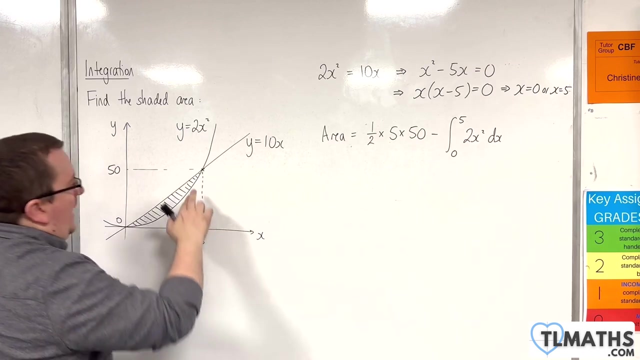 Okay, So that will leave me the shaded area that I want. So if you're a little bit puzzled as to why we're taking it away, Just recognise that that is the area of the triangle. This is the area underneath the curve, So all that area there. 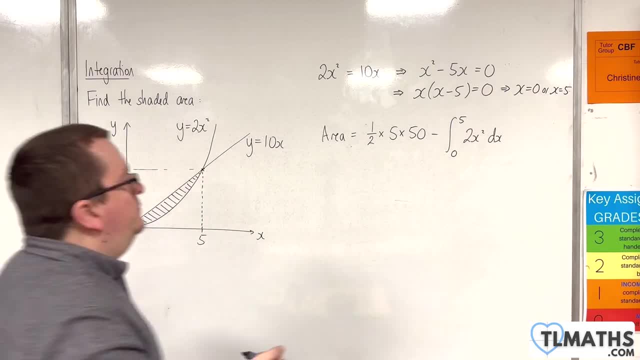 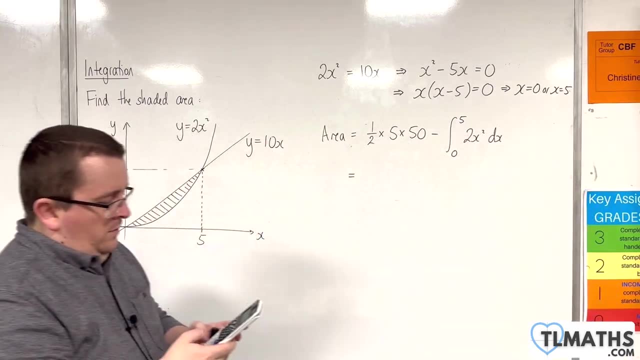 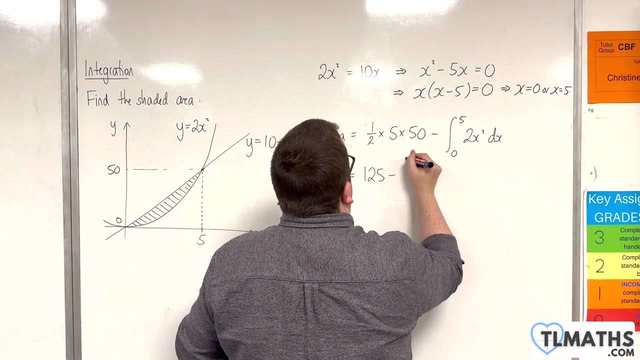 Okay, Which I'm going to take away from the area of the triangle. Okay, So we have 0.5 times 5 times 50. So 125.. Take away Now add 1 to the power divided by the new power. 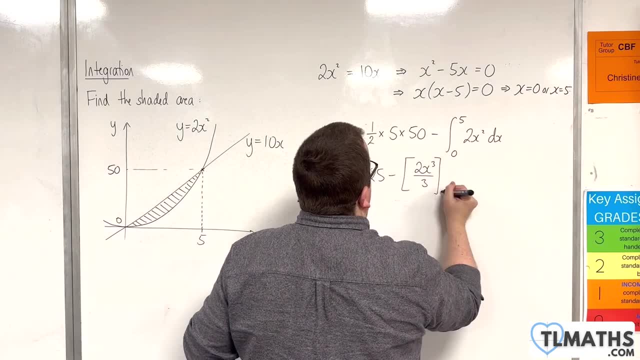 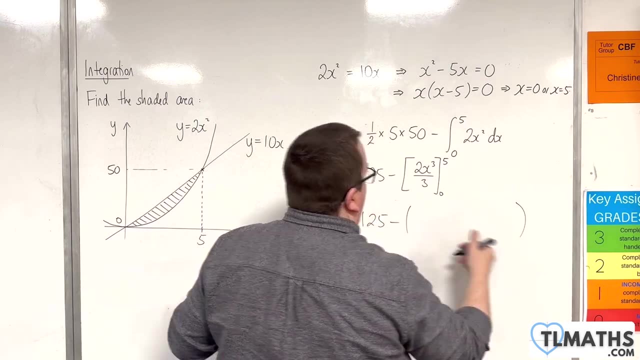 So 2x cubed over 3. Evaluate it between 0 and 5. So 125 take away. Now I'm going to open up a big bracket to include the evaluation of this, Just so I don't kind of get minus signs mixed up. 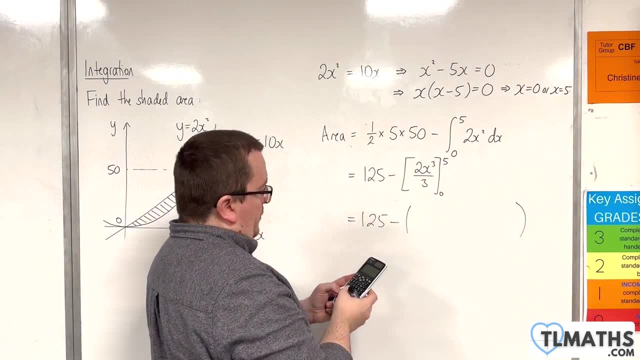 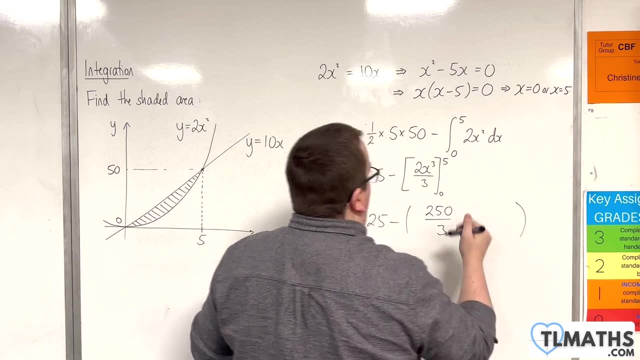 So substituting in 5. We're going to get 2 lots of 5 cubed Divided by 3. So that's 250 over 3. And then substituting 0. I'm going to get 0.. 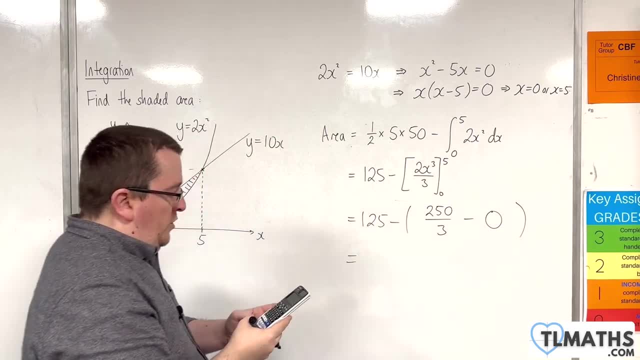 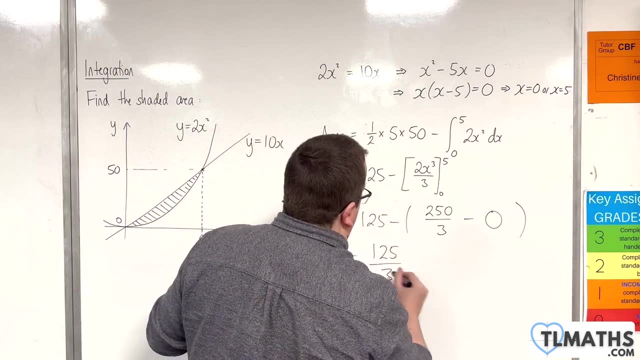 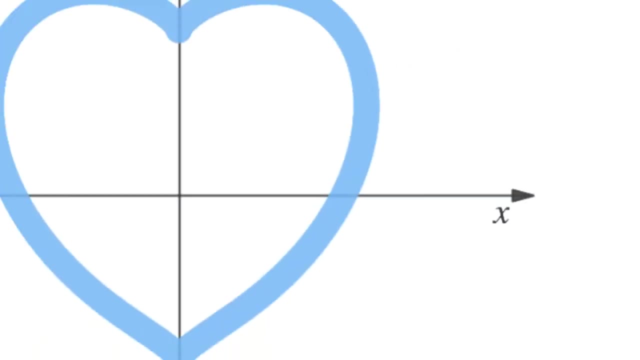 So that's what I'm taking away. So we have 125.. Take away 250 over 3.. And that is itself 125. Over 3.. Okay, So that is the exact shaded area that we needed. It's a very long day. The outside is going to be a lot more crowded. I'm just going to use a little bit of tape. I'll stay for a moment. It's just great to have you, But you know I've been a bit sad, you know. because every time we try to San Diego, You know these are, These are the crossings. This is like the one that just happened. I feel like it's come a long way. So we're going to get a lot of wind tonight. And we're going to. We're going to get a lot of wind, So that's the most important thing that we can. We're going to get. This is going to get a lot of wind, So that's the final graph that we're going to get. We're going to get 15.. So 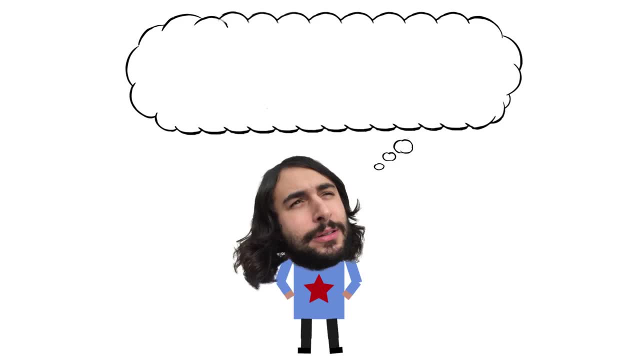 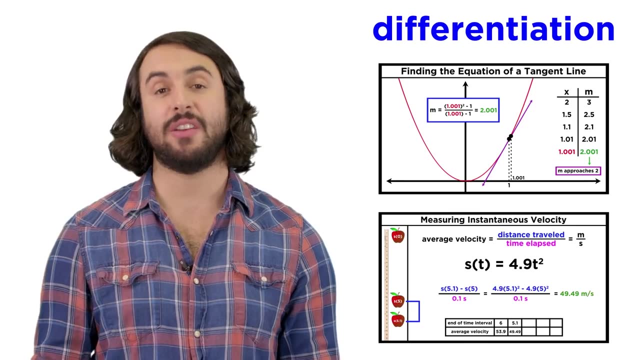 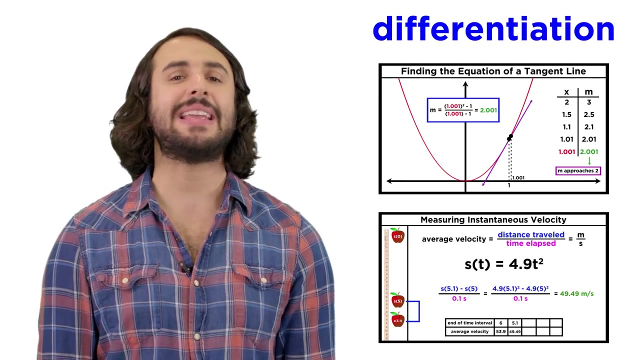 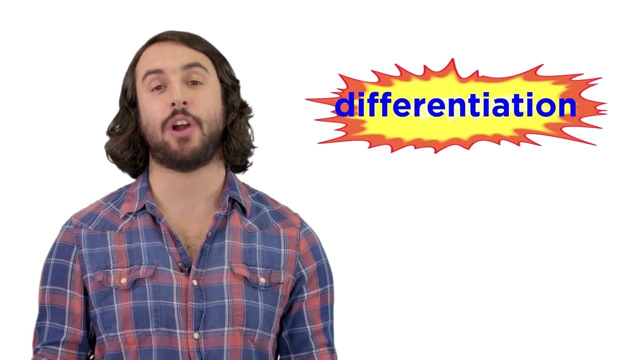 It's Professor Dave. let's define the derivative. From our earlier investigations with slopes of tangent lines and instantaneous velocities of falling objects, we gained a basic grasp of the concept of differentiation. So let's move forward and expand upon our understanding of this operation.